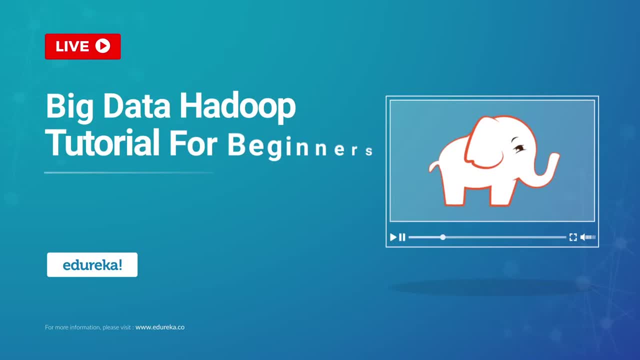 So good morning, good afternoon and good evening, guys, based on the time zones you all are coming from. So, guys, before we start with the session, can you all please give me a quick information, if you all can see my screen and hear me loud and clear as well. 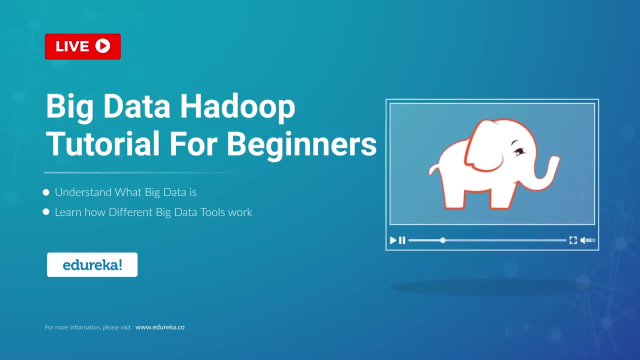 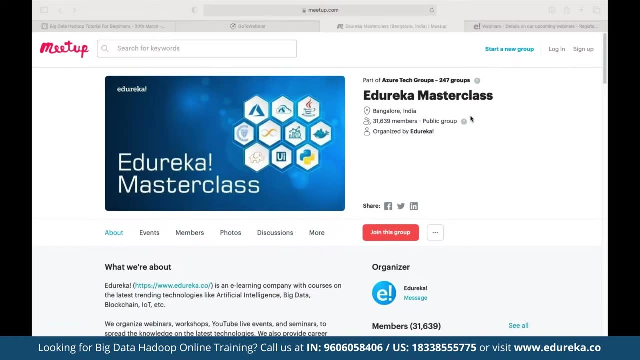 Perfect. Thank you for the information, everyone. So before we get started, let me quickly introduce Edutica Masterclass community with you all. So this community of masterclasses was started back in 2019, and since then we have been closing into almost 32,000 members. 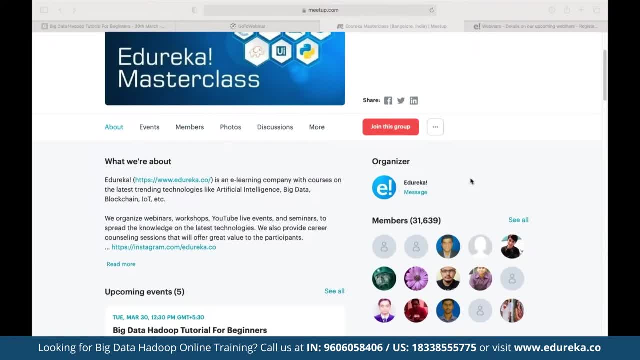 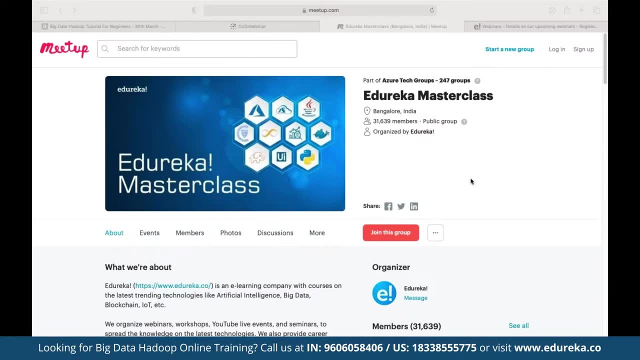 so far. So in these masterclasses, we conduct multiple webinars and live events on different topics, including blockchain, IoT, artificial intelligence and more. So let's get started. So the masterclasses, as you all know, is based on the foundation of the 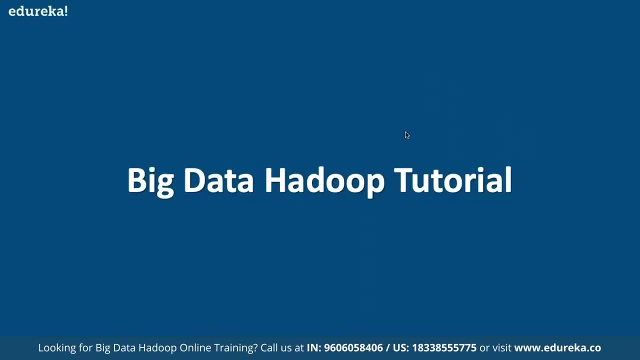 blockchain practice, And so we've developed a toolkit which is the most commonly used type of module in blockchainComeup, which is the main module. So that module covers nanotechnology, financial intelligence, machine learning, big data and multiple front end. and backend development technologies. And the best part about these seminars are they are absolutely free of cost, so there are no hidden charges involved here. So as a part of our discussion here today, we have gathered for our discussion on top of Big Data tutorials. So we have: we are going to discuss on the components of Big Data, what exactly it is, and then we are going to talk about what exactly is Big Data- Big Data as an opportunity, and then we are going to talk about the whole process of Big Data as an opportunity, and this will be. 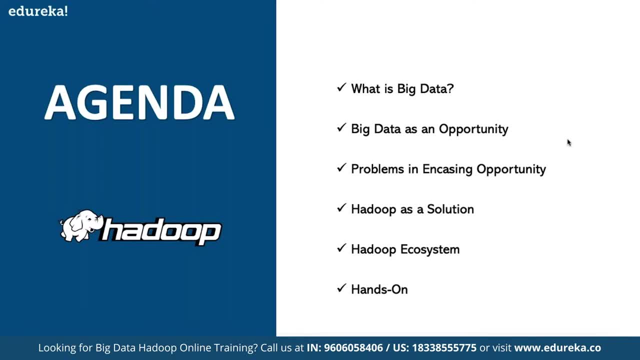 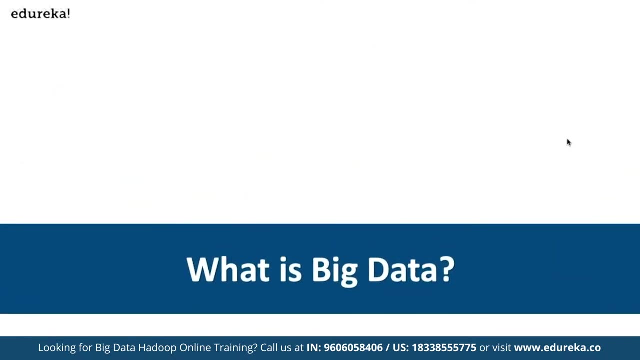 big data as an opportunity, and then the problems in encasing opportunity here: hadoop as a solution and hadoop ecosystem itself, and then we are going to talk about the hands-on, if possible. so basically, what exactly big data is. so big data is what big data in simple, in terms it's required for. 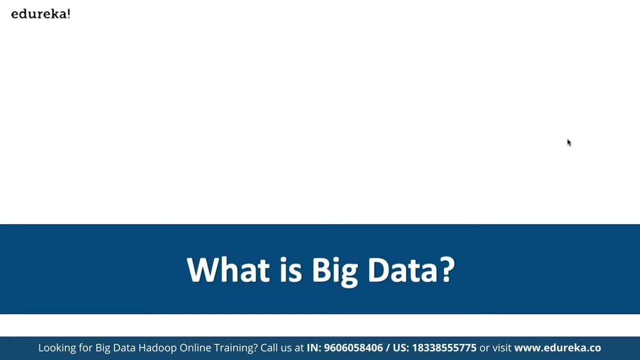 processing large amount of data. now for a project to be classified as big data, we need that project of having more than 1000 gb in size. then only it is going to be considered as a big data project, right? so any, any data size having less than 1000 gb is not going to be considered as a part of. 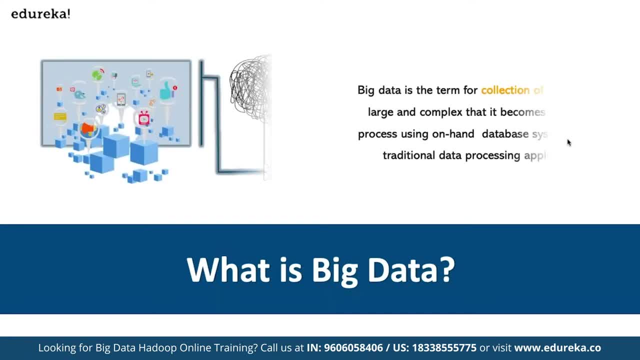 big data project. and big data is what? in simple layman terms, it's a process of reducing the time required for processing large amount of data set. for example, let's say, for processing we need, let's say, before processing, let's say, 100 gb of data, we need 10 days. so instead of doing that, 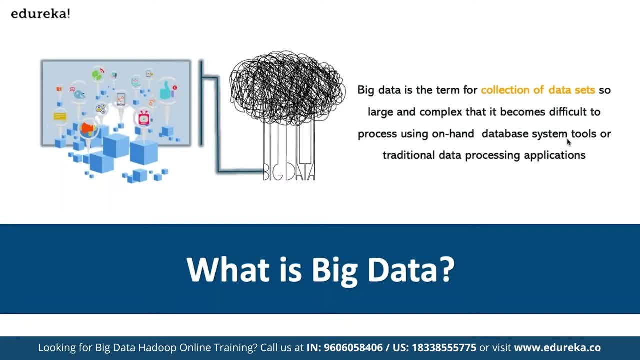 we can reduce the time here to to a few hours, to a few minutes as well, by using the concepts and the tools available under big data components. so that is exactly what it is. so, basically, if you remember the last time we had used floppy disk, right, so again, early we. 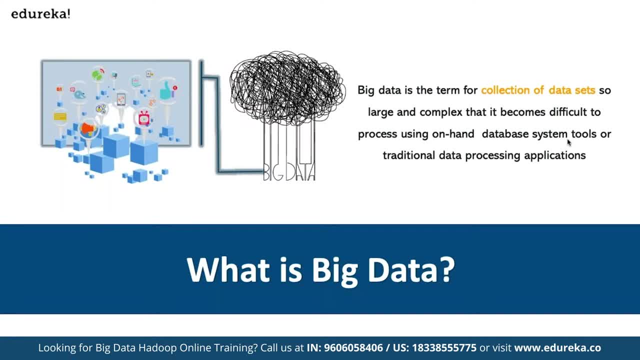 used to have floppy disks or a cd to store data, right, so let's say they were sufficient to handle the data amount of data at that point of time. but again now data is currently growing at an exponential rate, right, and that's why people are showing data in relational database systems. 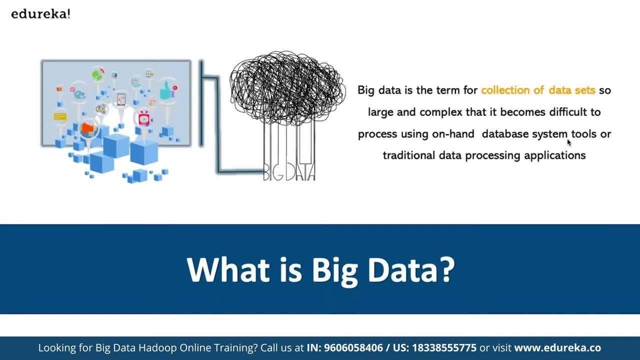 as well. but again, with the increase in the amount of data set now, the need for having a better insight of data is also going to be increased. that means now 80 percent of data is currently generated in terms of the unstructured data formats. that means when we say unstructured data, we mean 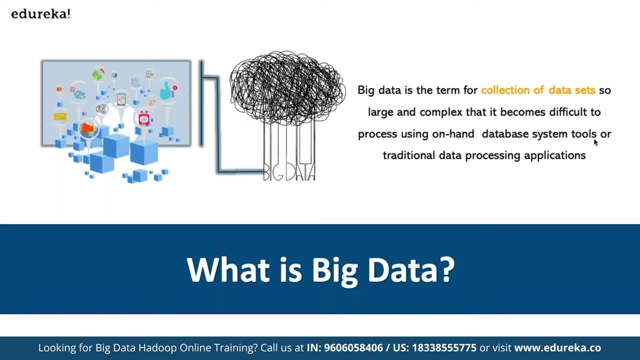 audio clips, video files, images, then these are considered as unstructured objects, and 80 percent of data right now is all unstructured thanks to all the social media platforms that we have, and that is what big data helps us in analyzing these kind of unstructured data set. so there are 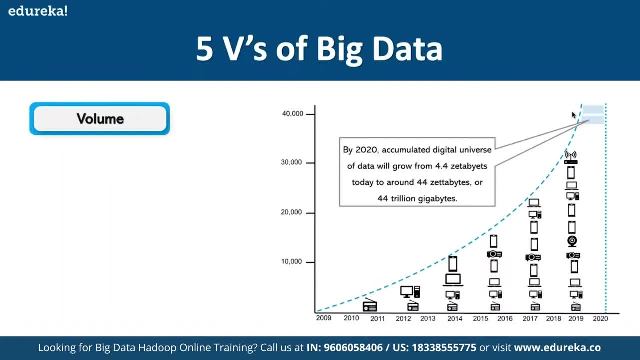 five v's of big data. we have volume. so by 2020, accumulated digital universe of data will grow from 4.4 zettabytes to create around 44 zettabytes or even 44 trillion gigabytes, as we can see here, and by next four years it is going to be increased to 100. 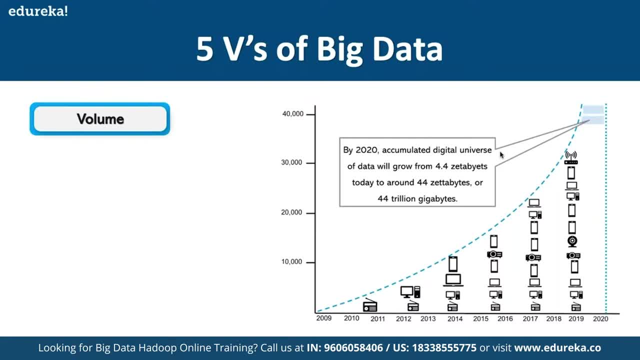 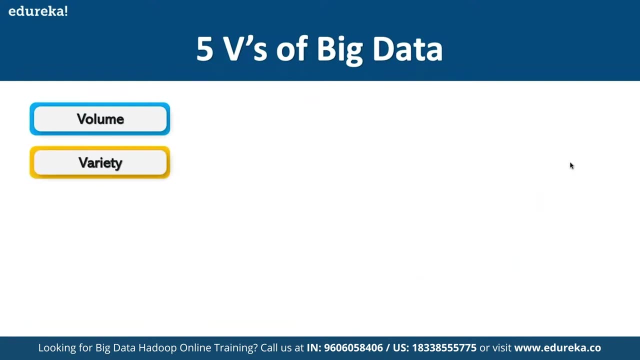 zettabytes on a per month basis, so, and that has been an exponential growth in terms of amount of data being generated on apartment basis, all thanks to 4g revolution, which happened back in 2016, and because from that point onwards, the data has increased multiples. right then, we have variety, so 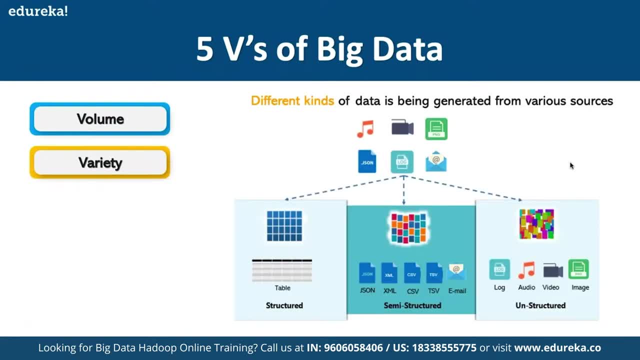 in terms of variety. we have to. so basically, here we have our data set up. so we have some data set up. focus the data in terms of different coming in different formats. so variety means what the data is in different formats. we have the structured database, we have the semi-structured, we have 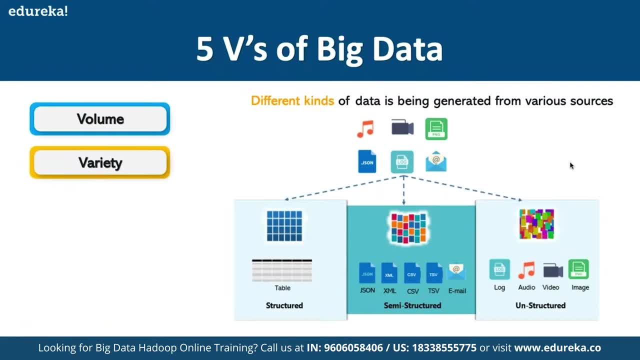 unstructured data set as well, correct. so, basically, in terms of all structured, we know we mean rdbl, we need dbms like databases. we have semi-structured, like we have emails, csv files, we have json scripts, xml files, and then we have unstructured, which is basically all the multimedia elements. 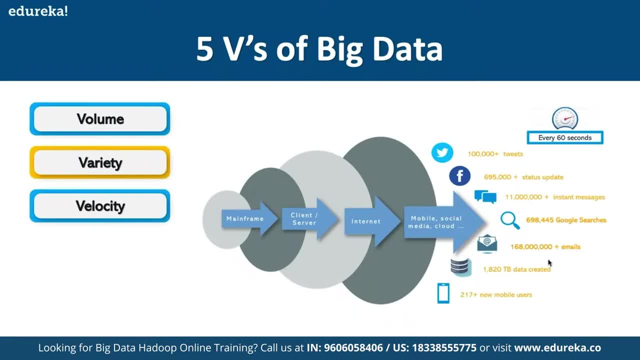 and then we have velocity. so velocity, that means the rate at which data is currently being generated. so we know, in terms of mainframe client server, internet, mobile, social media platforms, again, they all are generating humongous amount of data on a per second basis. they all are generating. 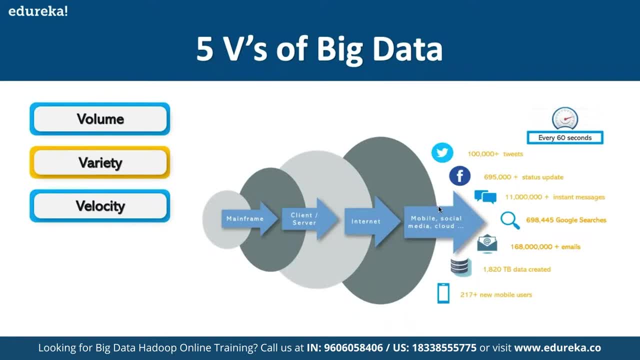 humongous amount of data on a per second basis, and that's why, again, in terms of the sales update here, in terms of the instant messages, We have to make sure that we do have the system to handle this much of data and that too. 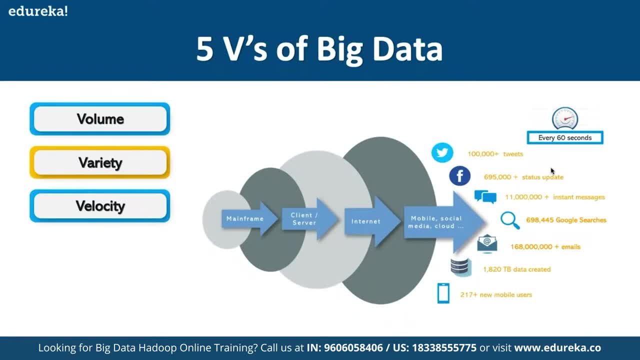 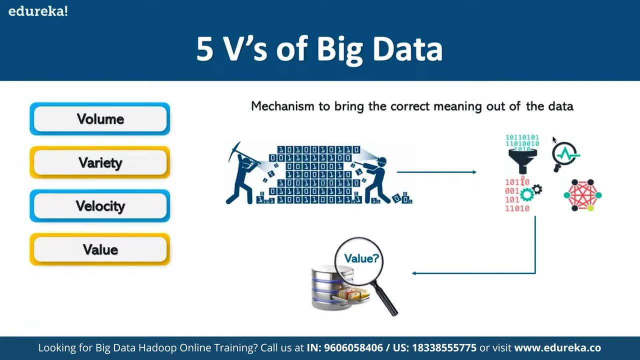 which is being generated at an exponential rate, And that is what, again, is handled by beta: the component itself, And here we have value. So, basically, when we are doing something, we have to first of all, before we start doing something, we have to evaluate: is that worthwhile? 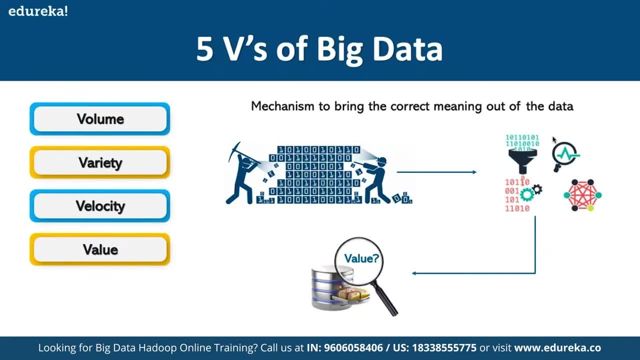 That means, if we are going to invest time in doing that activity, is it going to be worth it, Right? So, if that so, that is why we have to also evaluate the value. That means what is the value of data that we are going to follow? your value of information? 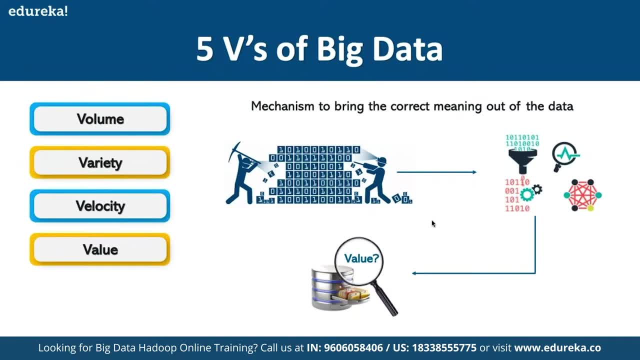 that we are going to get from this data set, If they, if the value is not going to be higher than the time and resource invested in solving and mining the data, and that, then then there is no use of big data there, right? So value? 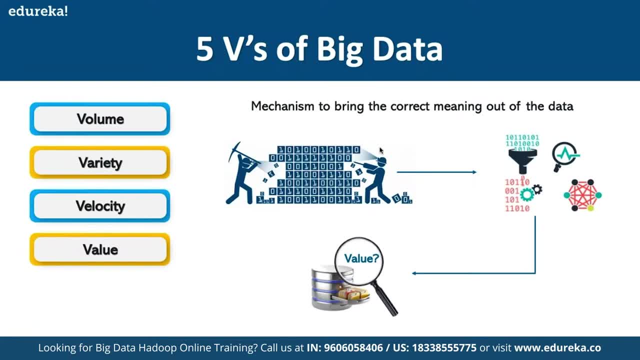 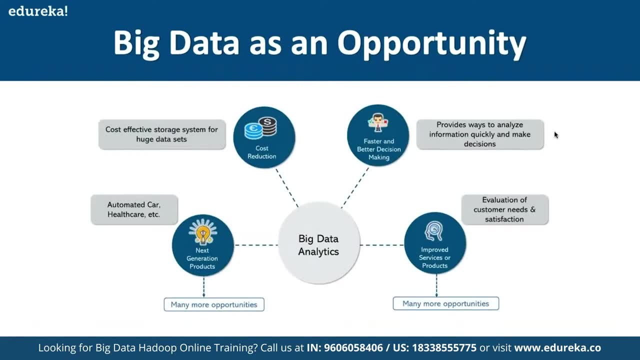 Has to be there, as it is not going to be feasible for us to mind the data right. So now we have big data as an opportunity. So big data, again analytics- is cost-effective because again it's so. it allows us to store, it allows us. 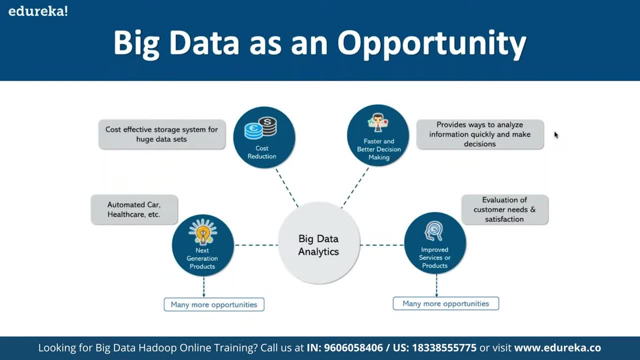 to so humongous amount of data set right. It has multiple opportunities in terms of the next generation of products because, again here, for creating something for the R&D part, We have to make use of multiple data, So like we have to take care of the data being generated. 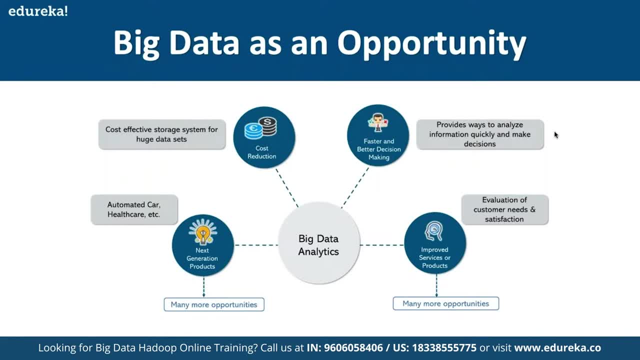 in automated, in automotive industry, in healthcare, where we have humongous amount of data already already just being there, and then we have to make sure we are able to provide ways to analyze information quickly and make decisions. We should be able to improve services and products. 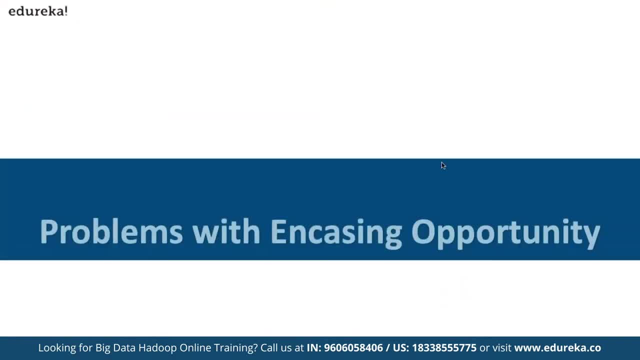 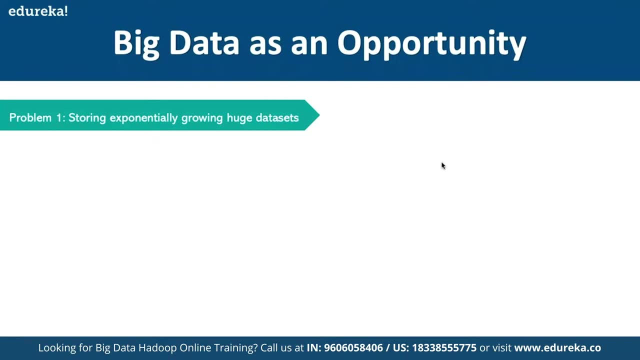 as a part of evaluation of customer needs. And now the problems with encasing opportunity. here is support. The first problem Is we have a huge problem in storing exponentially growing, huge data set. So data generated in past two years is more than the previous history in total. 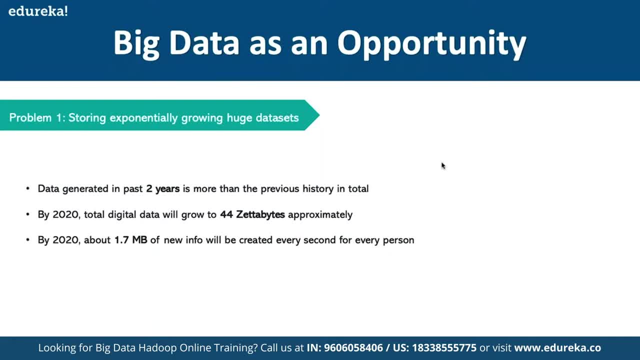 That's something to say. and again by 20, by again by the next day itself. So again, it is a story only. but again, by next two years it is going to grow more somewhere out, 80 zettabytes approximately, just maybe within next two years. 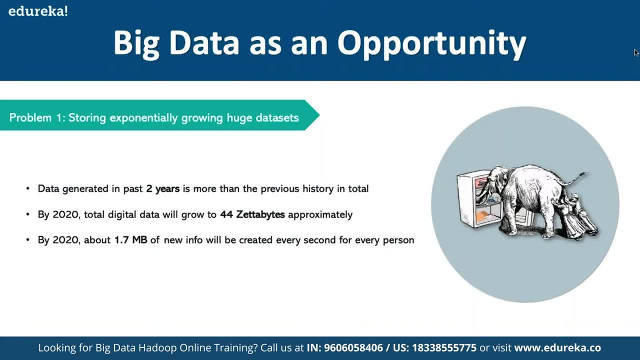 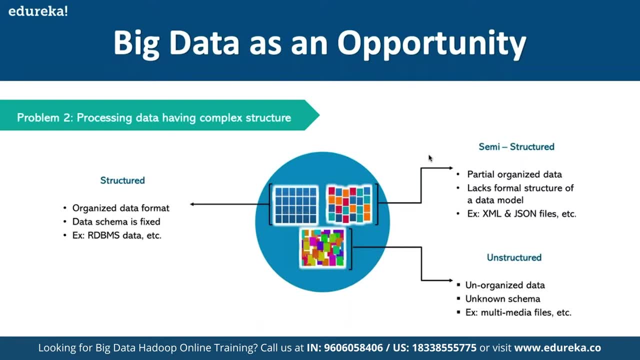 and that's why it has to be generated. And the second problem statement we have: it is going to be structured, for example. here We have to have a structure, organized format. That means data needs to be like in different formats in terms of RDP, nasita, sets here 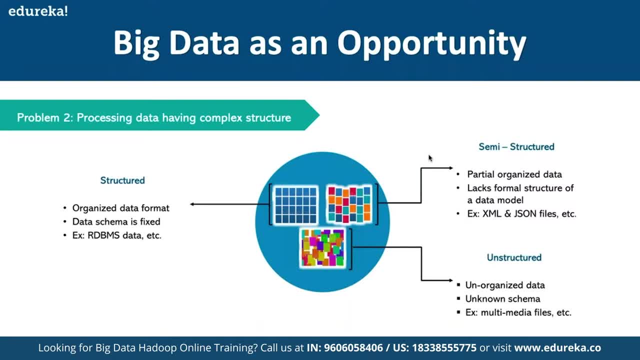 We have a fixed schema, whereas in terms of the semi-structured, we have partially organized data which lacks formal structure, and then, in terms of unstructured, We have all the muddy video files here. So now we need to have different ways of analyzing them and handling different files, and that is what we have. 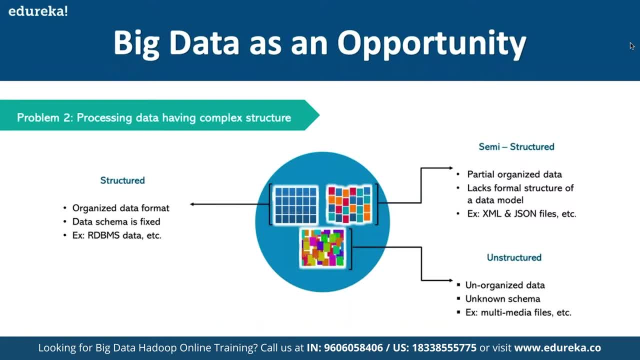 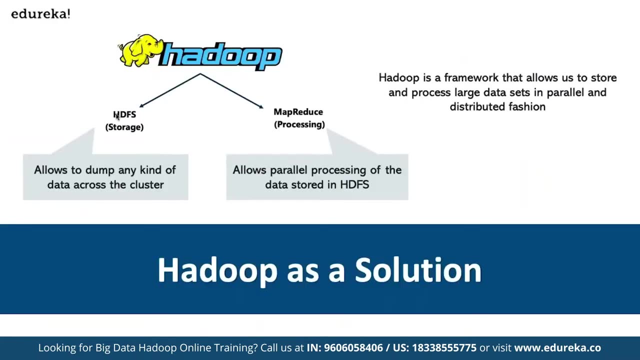 to make. that is what we have to focus on by using big data. So how? Hadoop is offered as a solution here. So basically, Hadoop allows us to dump any kind of data across the cluster and we basically has two main core components. We have our HDFS, which refers to Hadoop distributed file system. 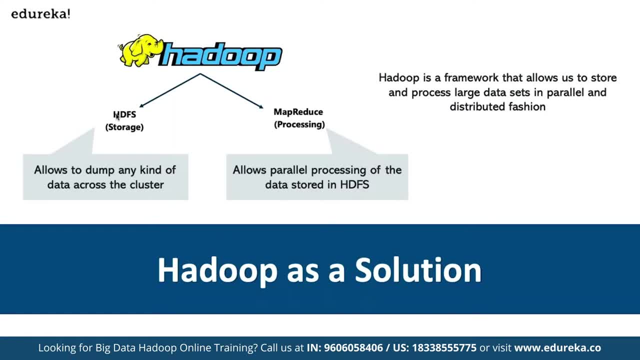 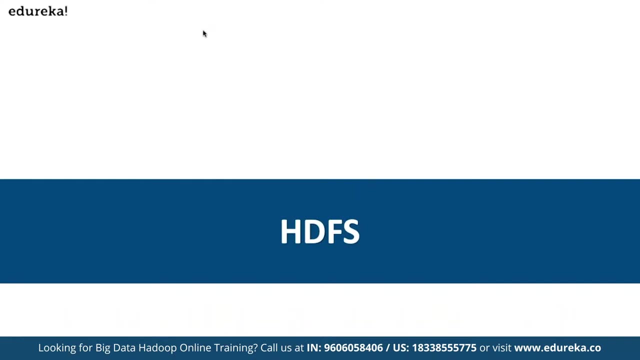 and then we have map reduce, which refers to processing, So it allows us to parallelly process the data stored in HDFS, All right. and then we have map reduce, So map reduce is basically used in combination with technologies, like we have Spark. 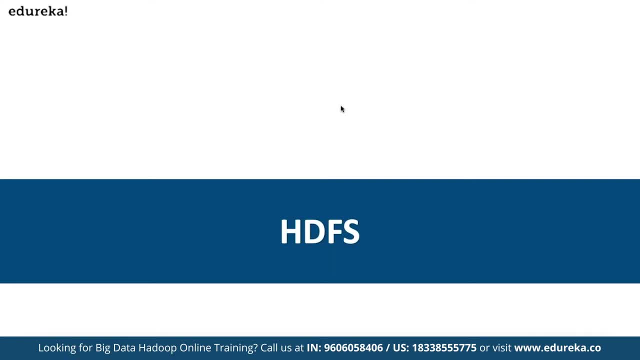 So Spark is basically used for giving us the access to a real-time processing of processing real-time stream of data. For example, we have to the streams, right. So that is what we can analyze by using the Spark streams. Let's discuss on that. 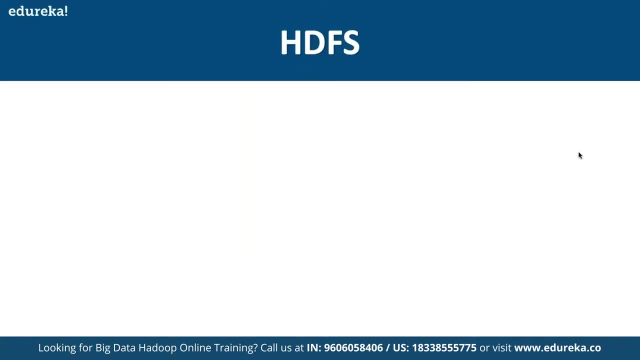 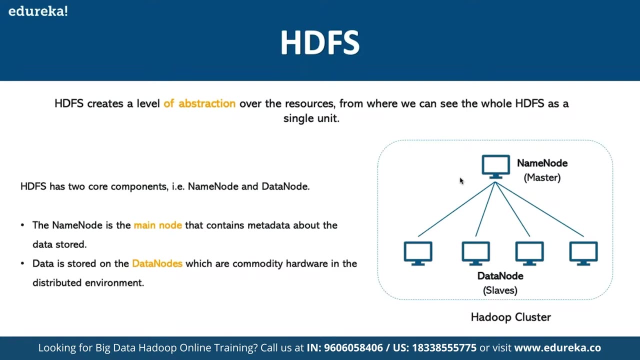 So here we have HDFS. So first of all, if you talk about HDFS- and HDFS is what it's- simply a distributed file system. So basically, here We can create a level of abstraction over the resources from where we can see the whole HDFS as a single unit and HDFS. 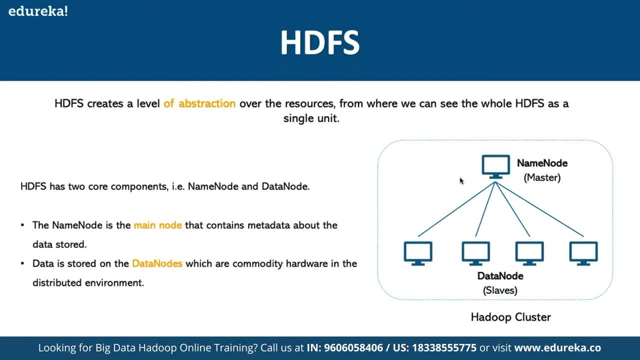 has two core components: the name node and data node. So name node is a main node that contains metadata about the data stored, and then we have the data node, which are simply commodity harvest in the distributed environment. So basically, under name node we can simply create multiple 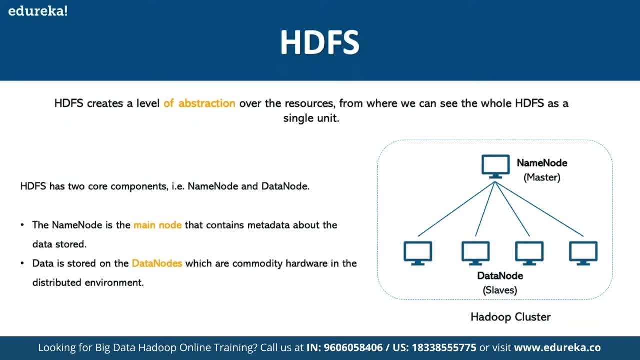 data nodes because at the end, processing is something that has to be done up in a cloud. We don't have. we are not going to do the entire processing in a single go correct by a single system, multiple systems. They all have to work parallelly to work on data processing and 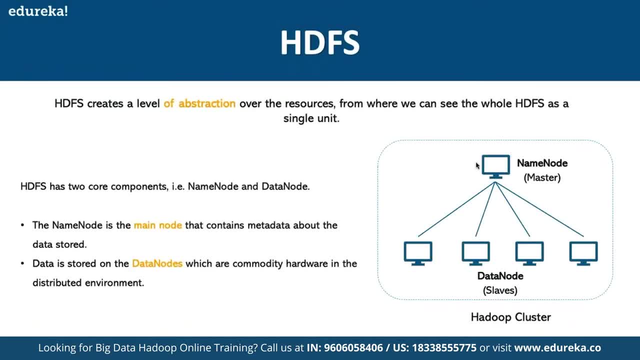 that is what is done by HDFS. here We have a master node with simply define- Okay, how many clusters are going to be defined, How many clusters are going to be created, And that's how it is going to work. So name node is a main node and the actual data is being stored. 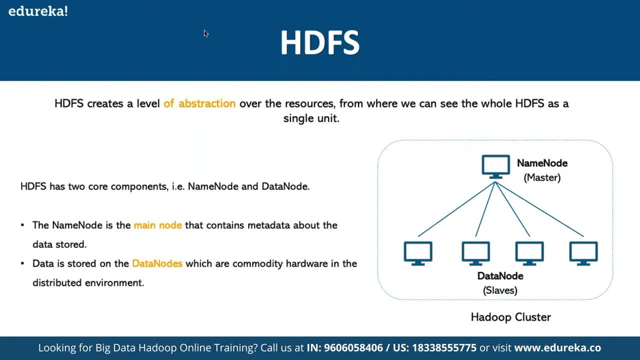 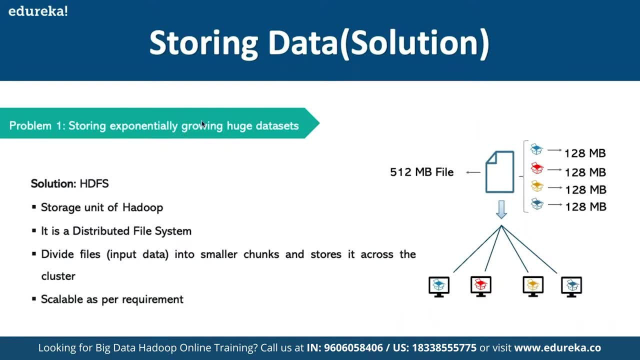 across different data nodes here. That's how it works, All right. So next we have to in data as a solution here. So when we talk about the main problem as storing exponentially growing, huge data set, the solution for that is HDFS, which is. 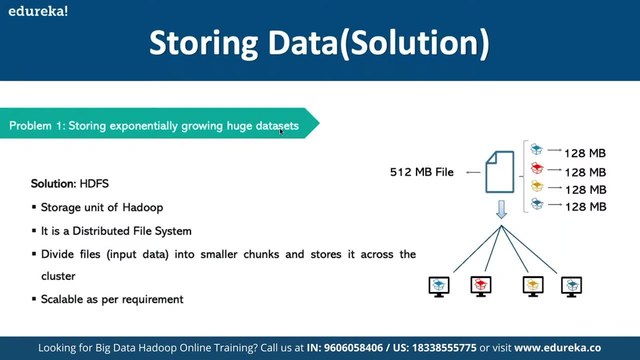 basically a storage unit of Hadoop. It is a distributed file system where we can divide files into multiple input data where we have a smaller chunk, and which sorts it across the different clusters and then we have scalable requirement. So basically, here we are going to take the requirement in. 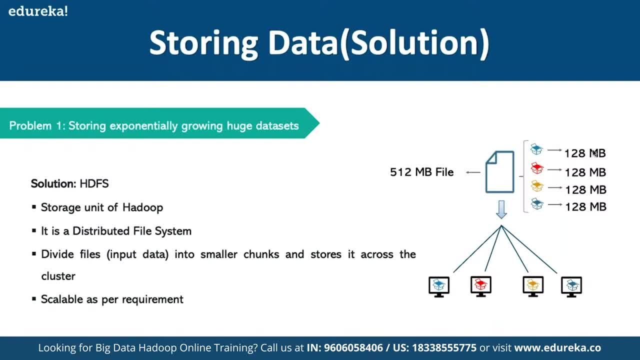 terms of the MB files, For example, here we have a large file as 500 MB files. So then we are going to divide this into smaller packages and then we are going to store it in different nodes so that we can process it as quickly as possible. 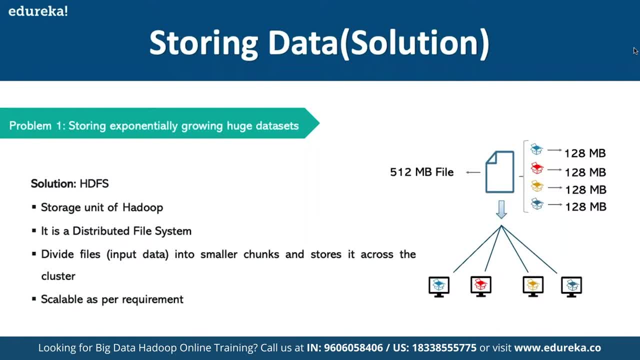 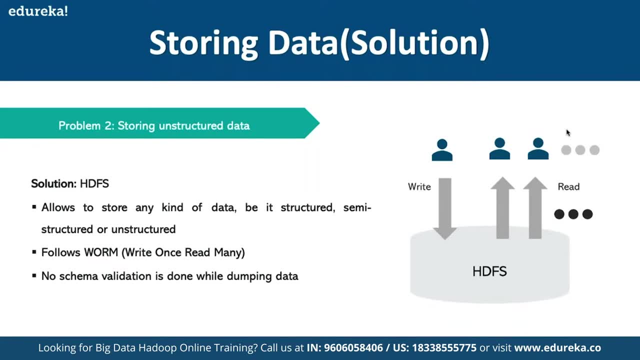 And then we have the second problem of storing the unstructured data. So how that is solved? by using HDFS. So HDFS allows us to store any kind of data, So it can be structured, semi-structured or unstructured. So basically, 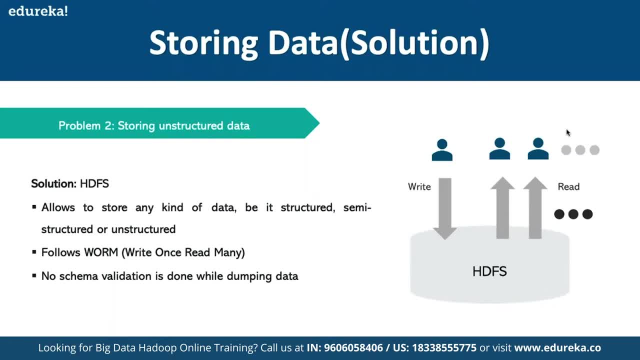 it forms the worm theory as in write once read many, So no schema validation is done while dumping the data set. So the users they can write data and again multiple read operations can perform on the data that has been written on HDFS. And third problem was processing data faster. 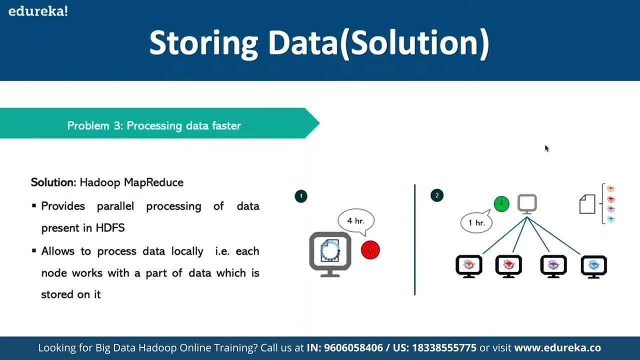 So the solution was Hadoop MapReduce. So it provides parallel processing of data present in HDFS, which allows us to process data locally. that is, each node works with part of data which is stored on it. So let's say, if we give a job to process thousand page to a, 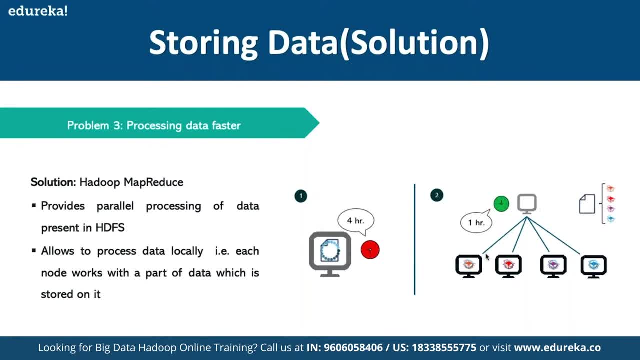 single system and we give the same job to another system where we have four connected systems and they all are having the capacity of going through, let's say, 250 pages on a per hour basis. So same job is going to take four hours for the system and the 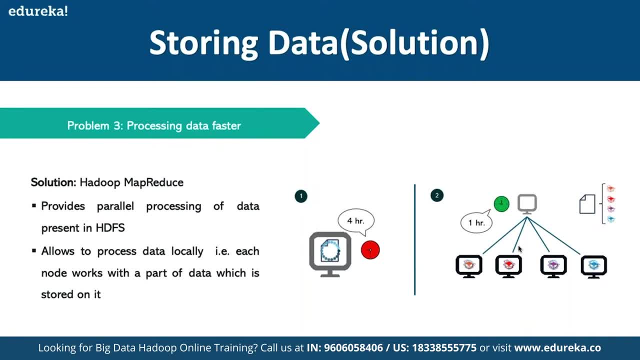 same job is going to take this one hour on the distributed system, because it seemed like the same problem statement that we have in mathematics back in our school. It is a one worker is able to complete a building and 30 days, and how many that? how much time will three workers take to complete? 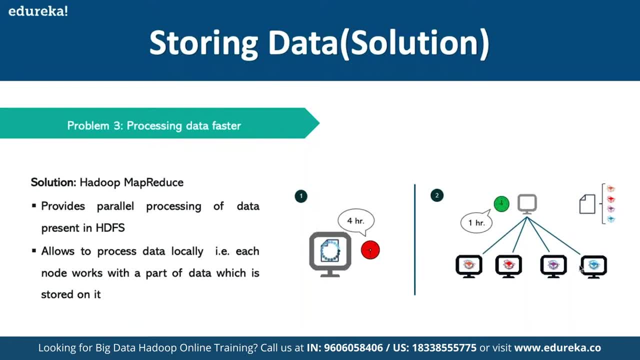 the same building right. So same thing is being done here. We are dividing the work into multiple workers so that it can work faster, and then we can get the output as quickly as possible. All right Now. next we have the Hadoop ecosystem. 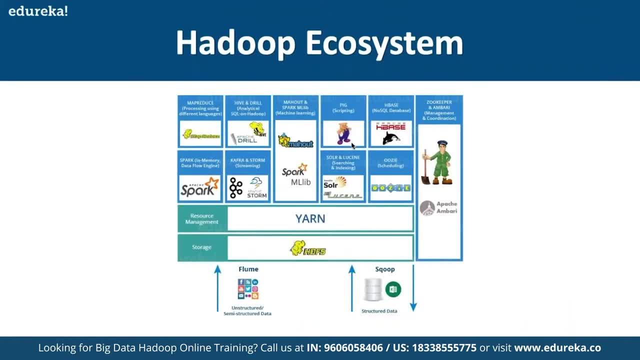 So, as we discussed, Hadoop is basically divided into HDFS and again we have multiple systems available under Hadoop. So here we have multiple components that we have MapReduce. So in MapReduce again we have. so basically MapReduce is used for a quick, we can say quick- batch processing and that is for 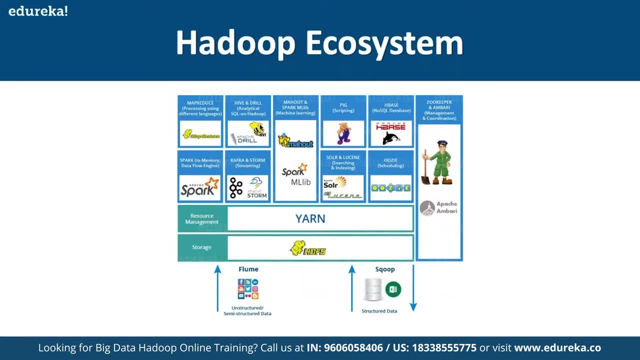 handling the real-time system the same way as Spark, and then we have the Kafka system, which is basically used as a message processing system along, which is meant to be used along with Spark. So basically, for flume is something that we use for the unstructured.